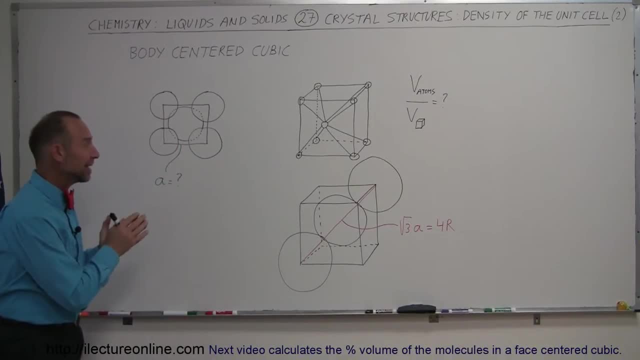 Welcome to ElectronLine, and here we're going to take a look at the density, the way the atoms are packed in what we call a body-centered cubic structure. We still have a simple cubic. we have a simple cube, but in this case not only do we have atoms at each corner of the cube, we also have one. 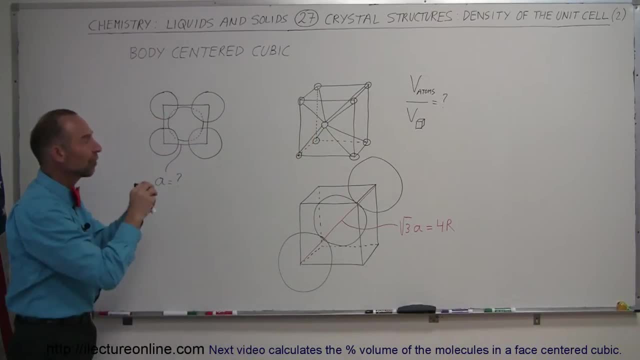 atom at the very center, body-centered as they call it, at the very center of the cube. So, first of all, how many atoms are now contained with this simple cube? And keeping in mind, of course, that because this atom at the very center, it pushes the four, the actually eight atoms right, there's the total. 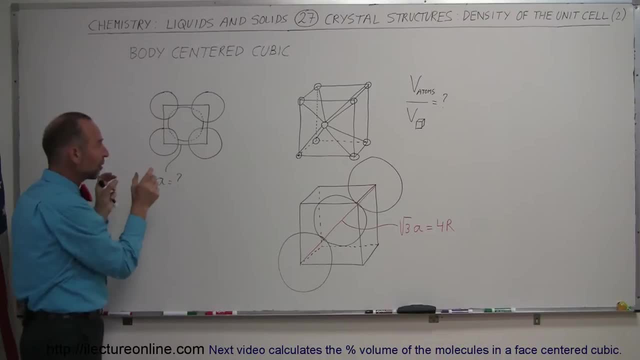 of eight atoms at each of the corner of the cube pushes them a little bit farther apart, where it's not likely that two will actually touch each other. right here, What's touching is the atoms that are at the corners with the one in the middle. The one in the middle is pushing the ones at the corners. 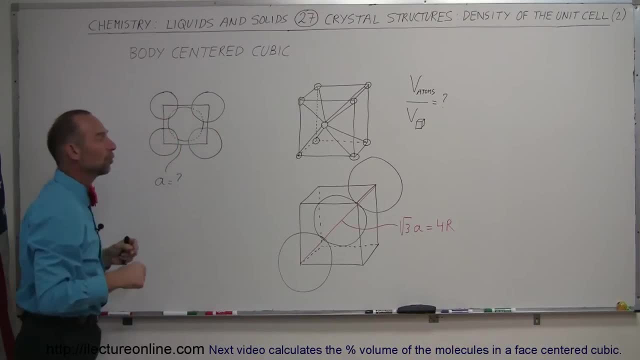 out a little bit and there's probably going to be some gaps between those atoms. So how do we find the density of this kind of packing? Remember the density when we only had atoms at the center, At the corners in the previous video, when those were all touching to each other. the volume was 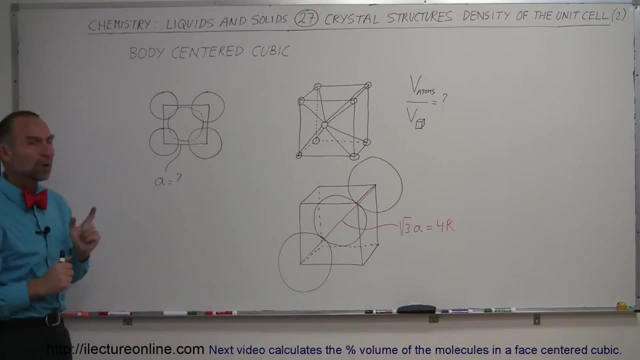 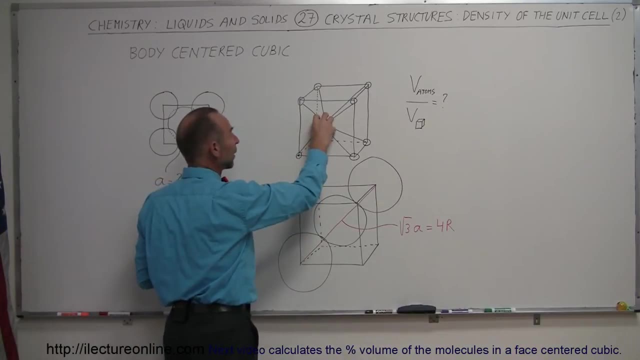 52 percent for the atoms inside the cube. Well, let's find out what the density is for this particular cube. First of all, what are the number of atoms inside? We'll definitely have the complete atom right here, and we still will have one-eighth of each of the eight atoms at each corner. 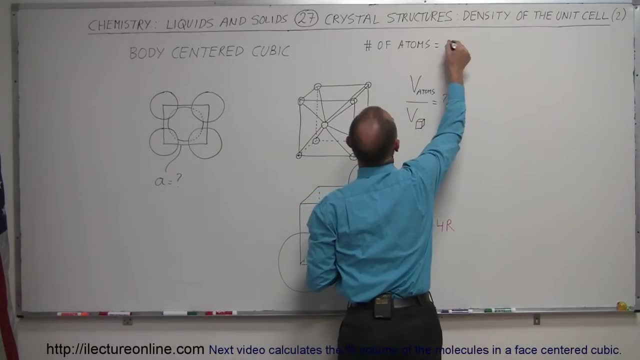 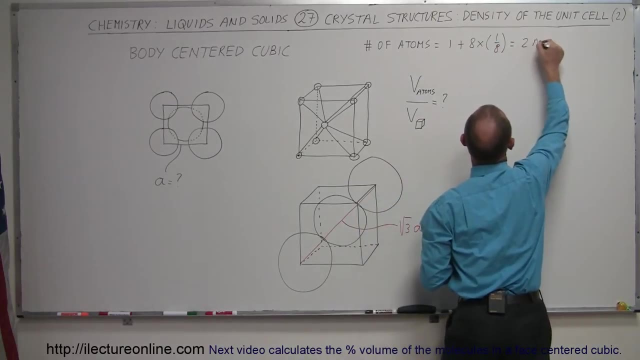 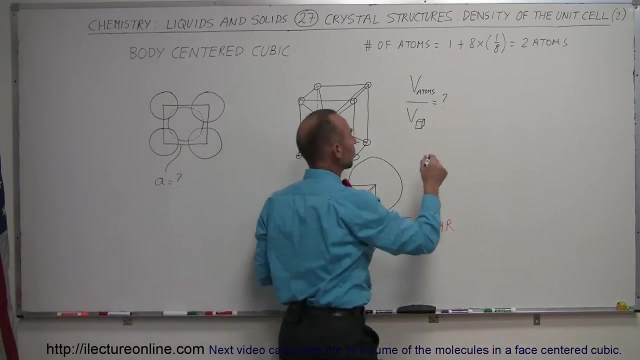 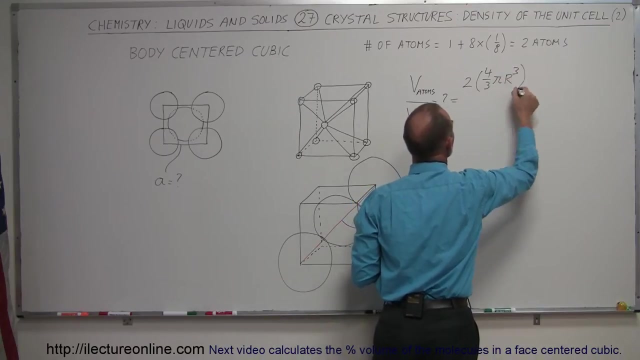 So the number of atoms will be equal to one plus eight times one-eighth of an atom, which is a total of two atoms. Therefore, the volume occupied by the atoms inside the cube will therefore be equal to two times the volume of a single cube, which is four-thirds pi? r cubed. All right, 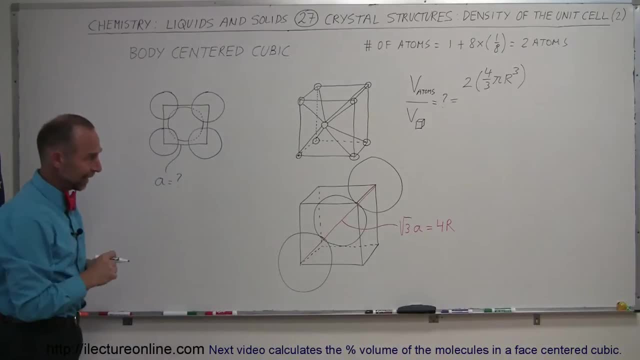 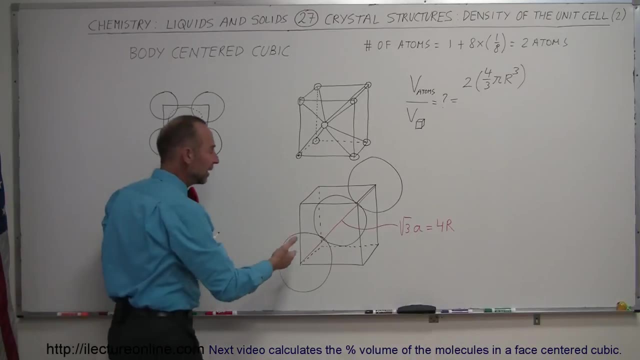 so that will be the volume of all the atoms inside the cube. Now, what is the dimension of the cube? Well, the only way in which the atoms touch is across the diagonal line from the front left corner to the center. By the way, the volume of atoms at the corners will have to be too much. 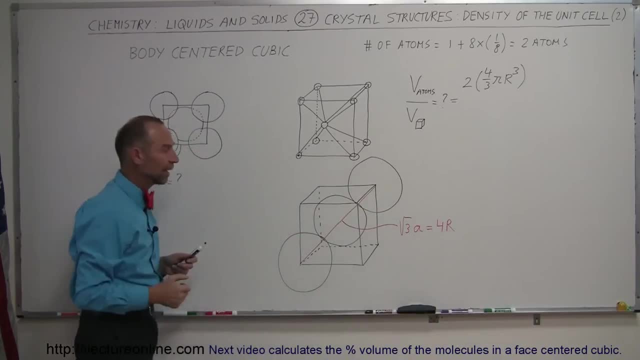 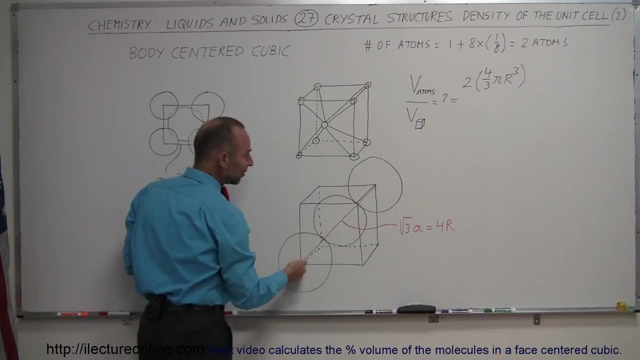 the back rear corner, or to the right rear corner, I should say. So that means that if we draw a line from the front of this corner here to the back of that corner right there, that distance is equal to the cube root of three times the side, If the side is equal. 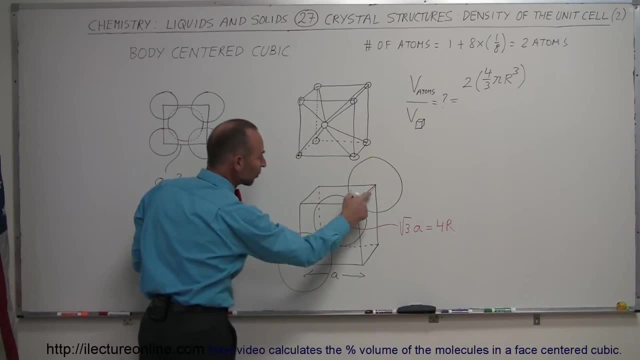 to A, then the diagonal from one corner across to the other corner, like that, is the square root of three times A, And that will then have to be equal to four times the radius of an atom. I have one r here, two r, three r and four r, So the cube root of three times. 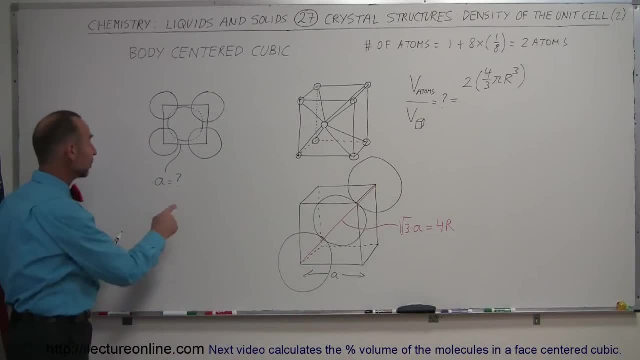 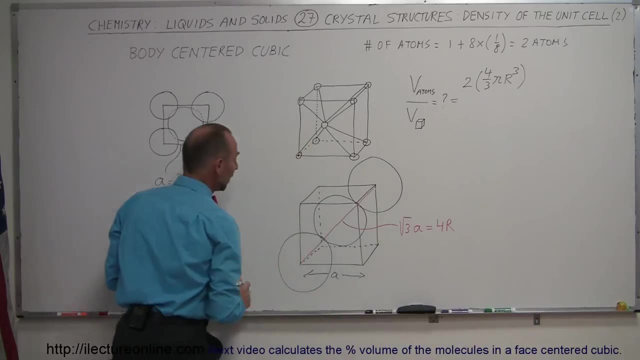 the side equals four times the radius. From that we should be able to find out what the side is in terms of the radius. So all we have to do is divide both sides by the square root of three and we get. A is therefore equal to four divided by the square root of three. 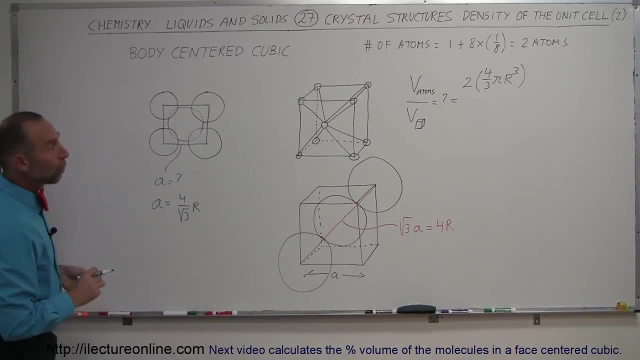 times r, Or I guess we could replace r by terms in A. That might even be a better thing to do. What we could do is rearrange this and say that r is equal to the square root of three divided by four times A, Simply by moving the square root of three up here and the four 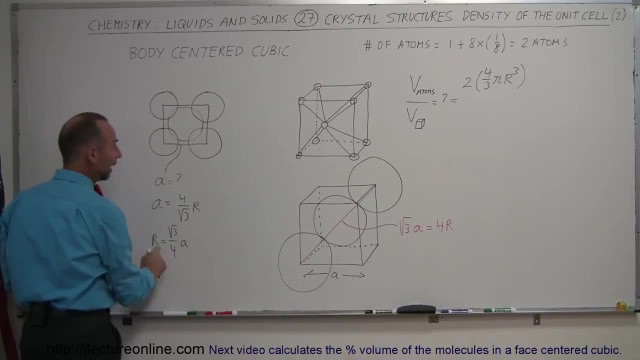 down here we get the square root of three. divided by four times A equals r, And that can then be replaced or substituted in this equation right over there. Alright now, also keep in mind that the volume of cube is going to be A cubed, So this is: 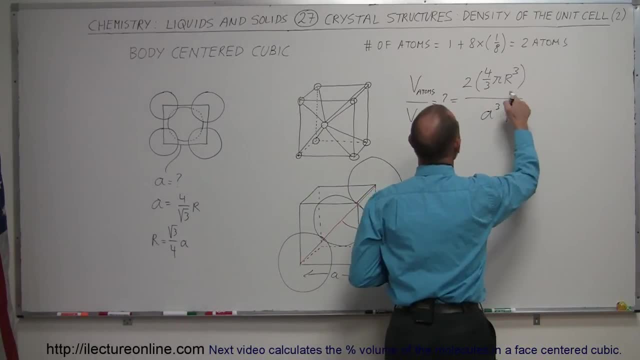 this number here divided by A cubed, Turning this into A's. what we could do is simply replace r by this quantity right there and multiply the two times four, bringing the three down here, so we have this equal to eight pi divided. 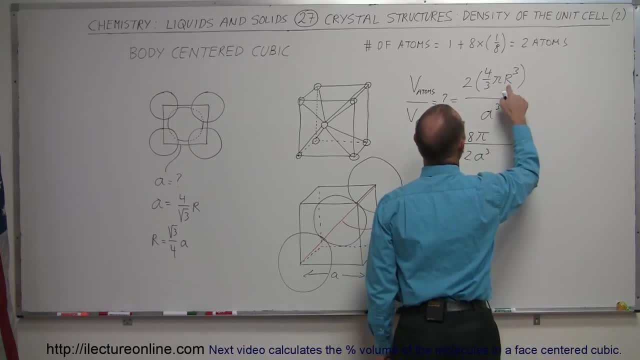 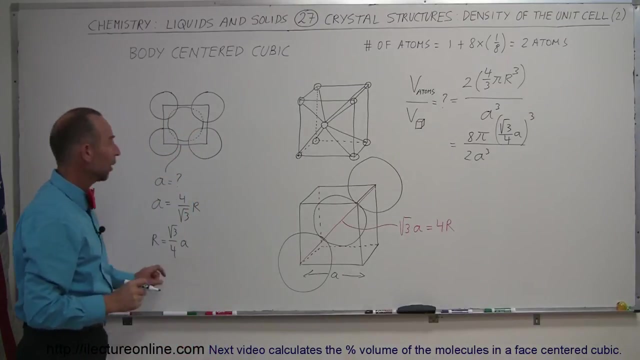 by two A cubed, And instead of r- cubed, we're going to write this quantity cubed. So we have the square root of three divided by four times A quantity cubed. Okay, so we simply replaced r by what r is equal to in terms of the side of the cube. 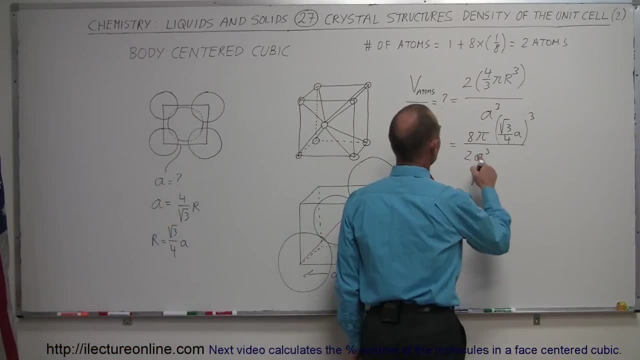 Okay, continuing on. A divided by- oh, this should be a three, not a two. Two times four is eight. divided by three, this should be a three. right there, Alright, continuing on. So we have eight pi the square root of three. cubed, that would be three times the square.